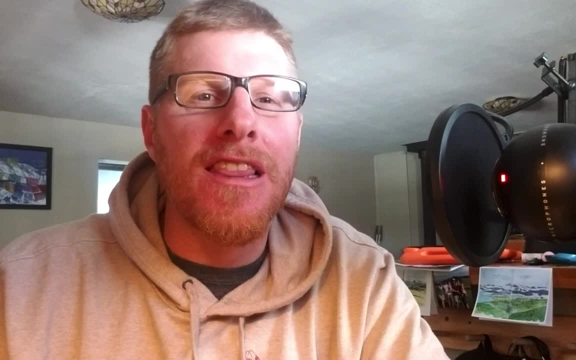 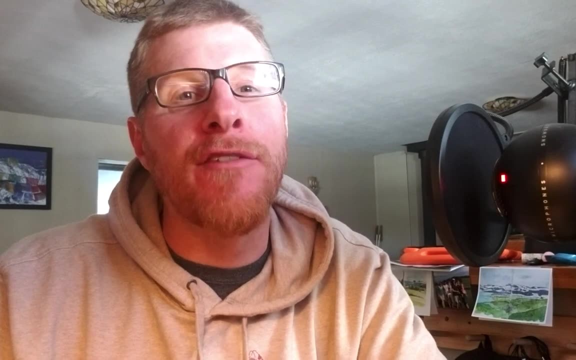 Hey there, econ students and teachers. In this video we're going to define what the labor force is in a nation and learn how to calculate the labor force participation rate. Thanks for watching. Please subscribe to my channel and head over to econclassroomcom for more resources for economic students and teachers. 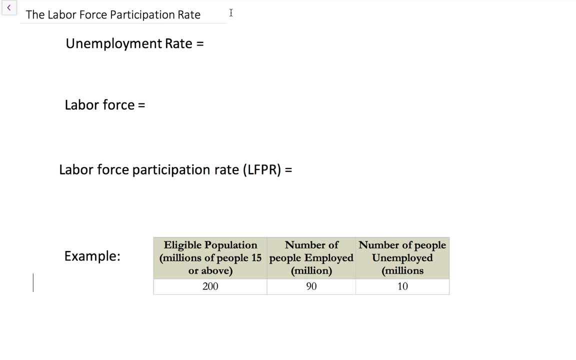 In this video, we're going to talk about the labor force and the labor force participation rate. We need to know what the labor force is because we need to be able to calculate the unemployment rate, something that you're always going to have to be able to do in a macroeconomics course. 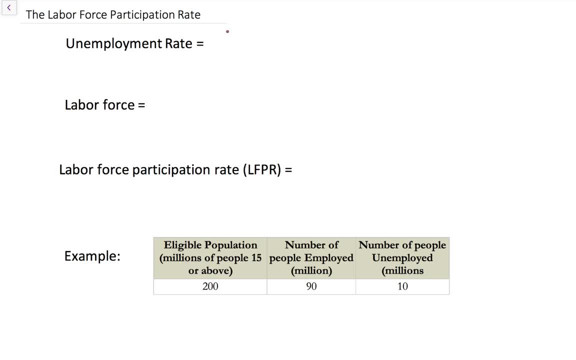 So let's review what the unemployment rate measures and then we'll move on to define the labor force and the labor force participation rate. The unemployment rate, you'll recall, is calculated by finding the percentage of the total labor force TLF that is unemployed. 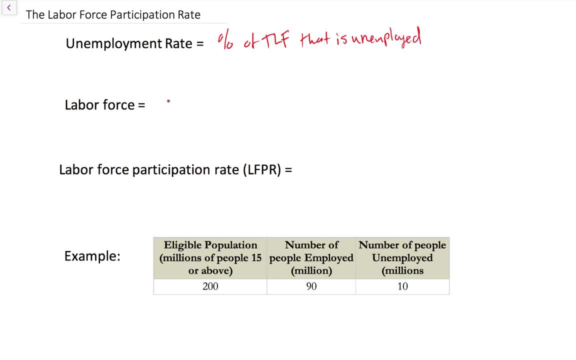 So that raises the question: what is the total labor force? What is the labor force? The labor force is defined as the economically active population. It includes both the people who are employed or unemployed. In other words, to be part of the labor force, an individual must either have a job, either a full-time job or a part-time job, or must be actively searching for a job and unable to find one. 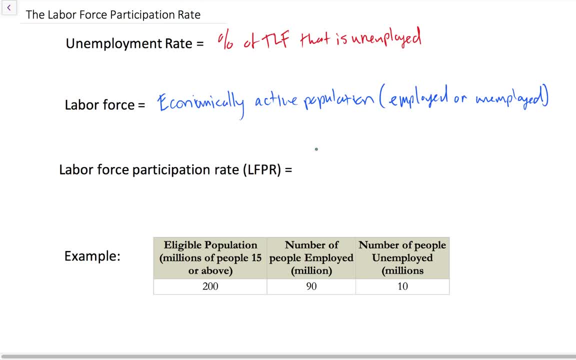 So that raises the question: what is the total labor force? What is the labor force? The labor force is defined as the economically active population. So the labor force participation rate is the percentage of the adult population in a country that is economically active. It is defined as the number of people employed plus the number of 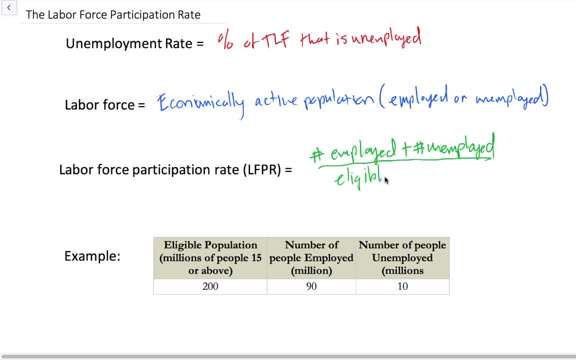 people unemployed divided by the eligible population, which in most countries is 16 and above. Now, not included in the eligible population are some individuals such as those who are institutionalized as in they are in prison or in active duty, in other words, part of the military. 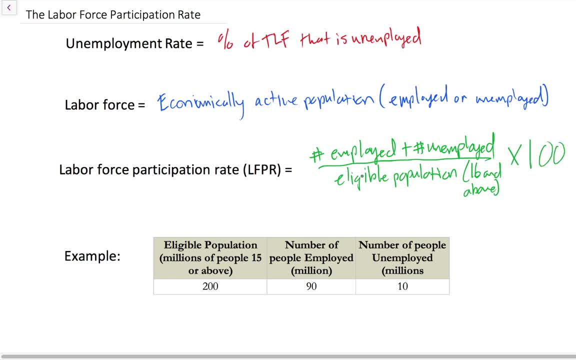 So we're finding the total percentage of the eligible population that is economically active. That will give us the labor force participation rate. Let's do an example down here. We have a country with a population of 200 million adults. These are the eligible people who could be. 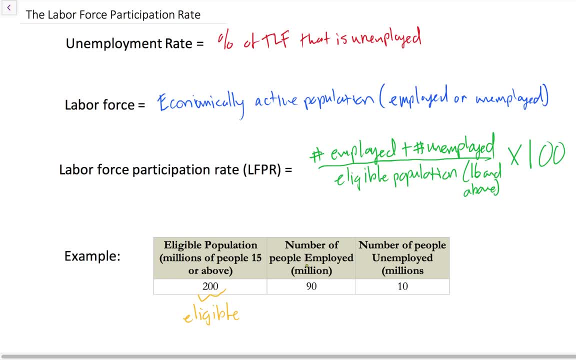 participating in the labor force. Of those, 90 million are employed. We've got 90 million people employed and 10 million people are unemployed. So this is the economically active population. We can now calculate the labor force participation rate and we'll be able to calculate the unemployment rate from this data. The labor